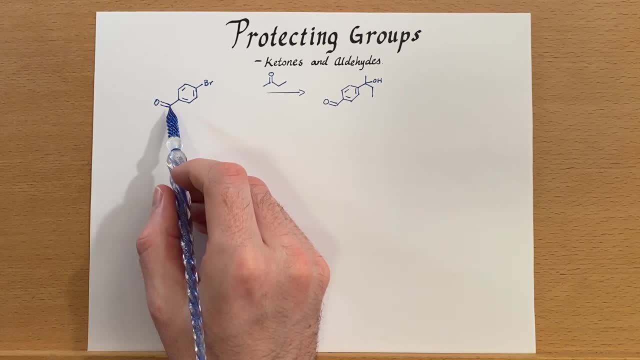 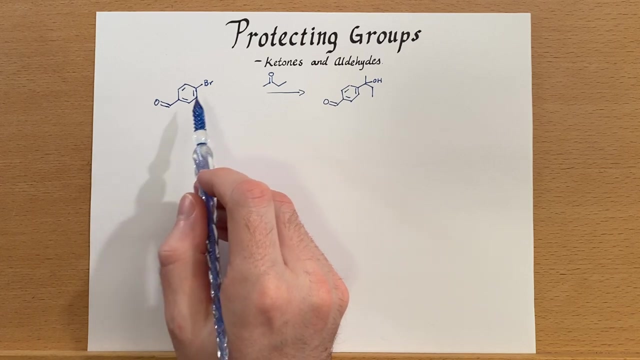 reagent, the Grignard reagent- It will react over here on a different one of itself and it will probably make some weird polymer in the process, and we don't want that to happen. So what we really need to do, instead of going directly and making a Grignard and then going here- 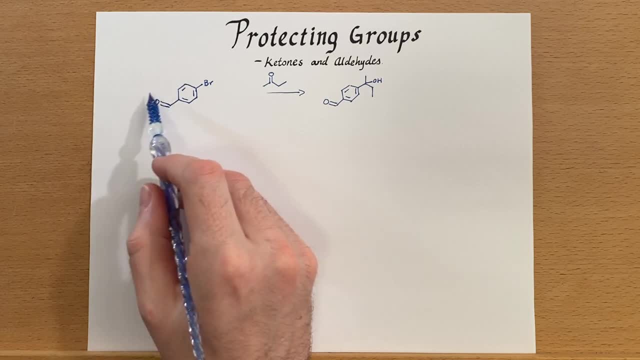 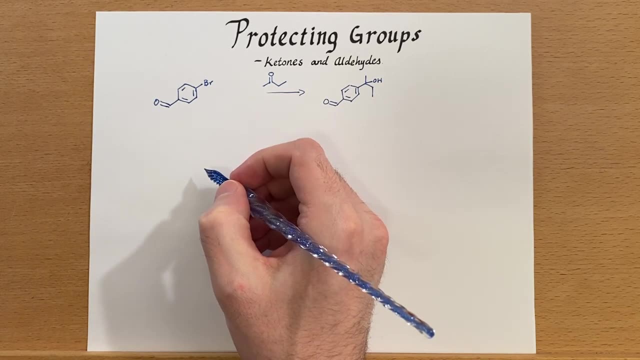 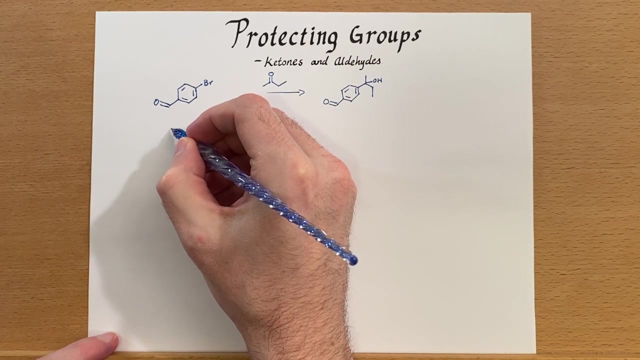 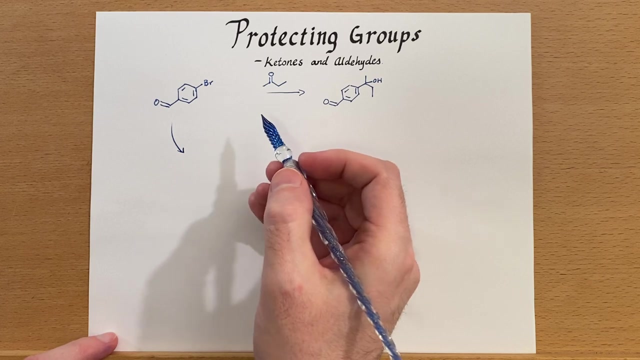 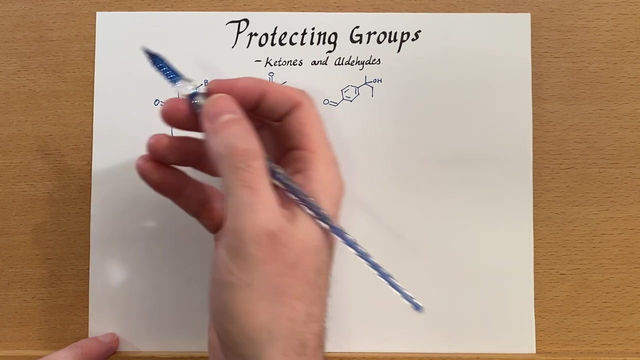 which will not work. we need to somehow protect this aldehyde. So one of the best ways to do that is to form it into an acetal. So let's do that And typically when people form the protecting group, now you can do the acetal actually with really any alcohol that you want, Like we could put. 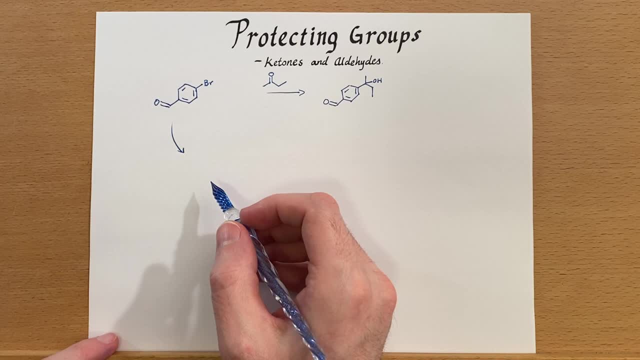 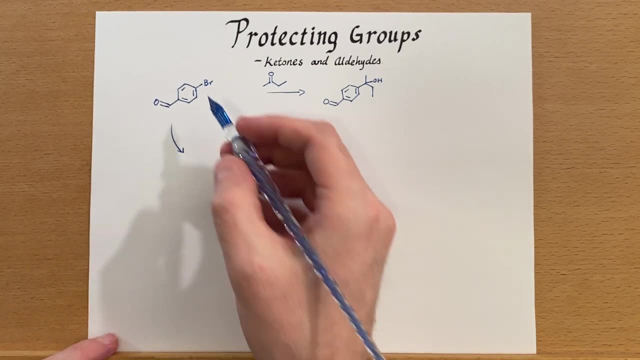 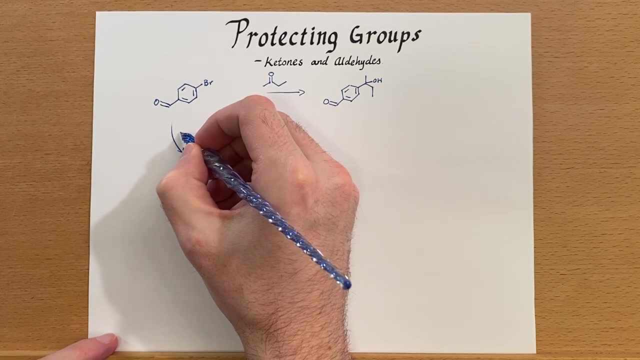 methanol in here and add sulfuric acid, put a lot of methanol in there, form the acetal out of that. But for the most part people like to use ethylene glycol because you only need one of them. 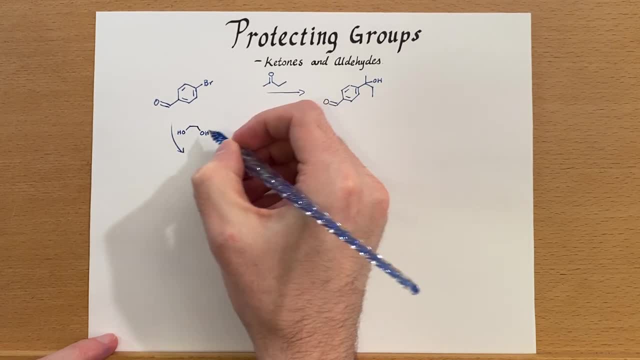 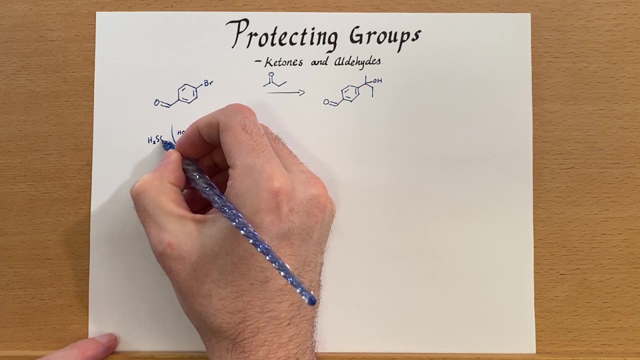 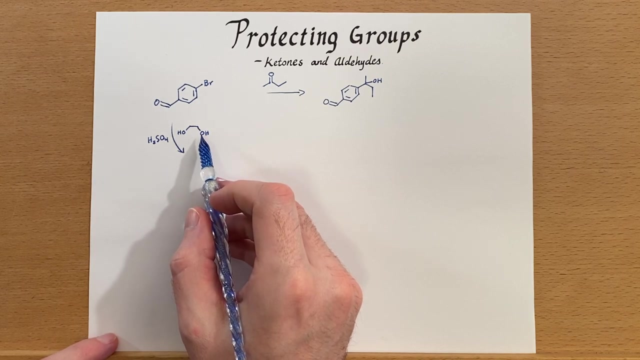 Because it has two alcohols on it and it makes a five-membered ring which is pretty stable and it's a little faster to form. This is also going to be a lower steric hindrance because it's all tied up nice and neat. So there's a lot of advantages to using ethylene glycol. So when we do this, we will form the acetal which looks like this: Still have the bromine on it. So now we have this acetal, which is a five-membered ring in this case. 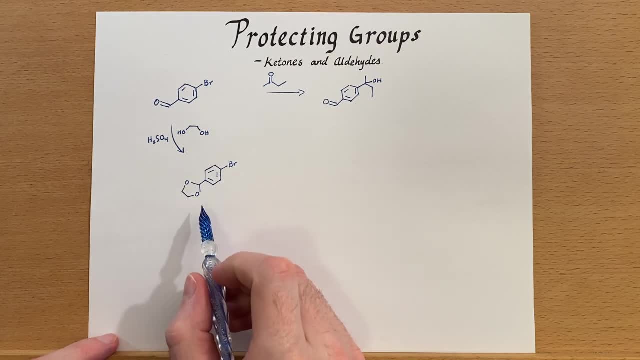 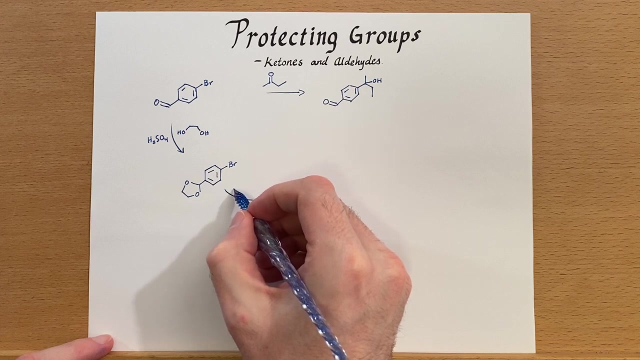 and it's protecting our aldehyde. now, when we make the Grignard, we will not. we will not have a reaction with the aldehyde. so we're going to add in solid magnesium and probably some THF or some other solvent like similar ether solvent, and we'll make sure this is a dry conditions and when we do that we'll be. 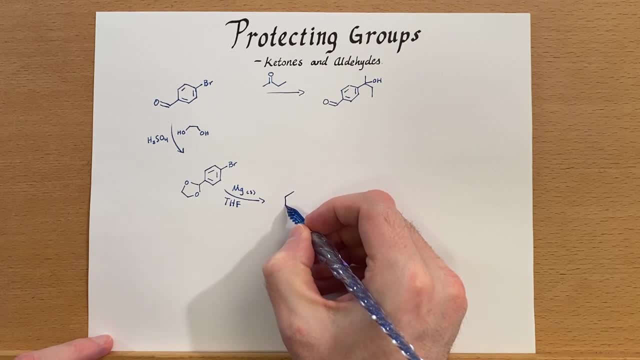 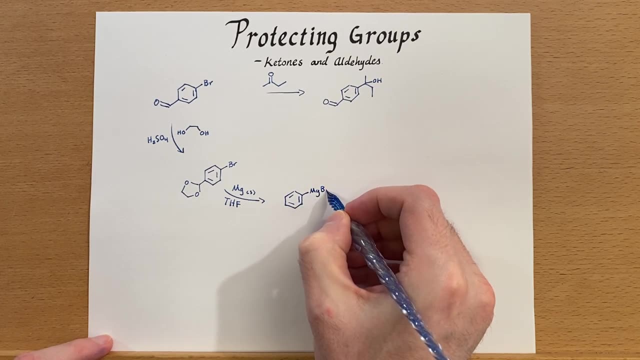 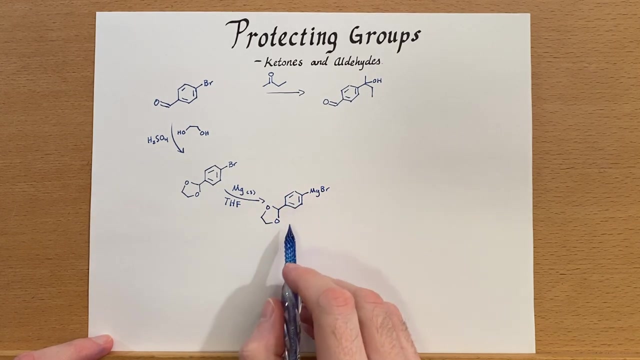 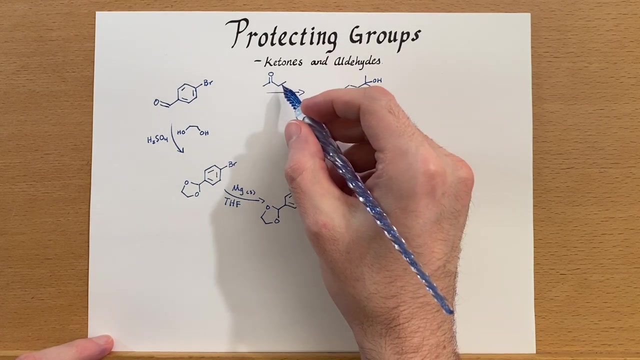 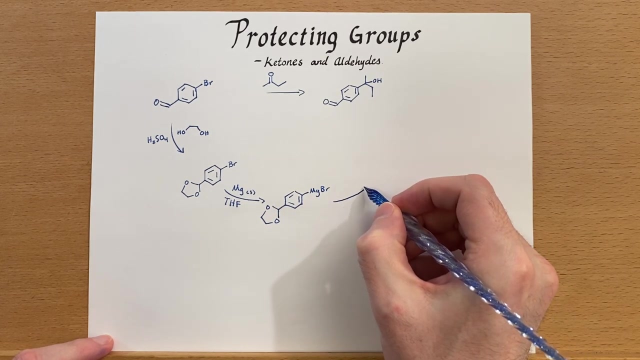 able to make our Grignard with the protecting group. now we have this protected. still, once we have that, we will add our ketone that we wish to have react with the Grignard and then we'll have to have a step one and step two. here is going to be 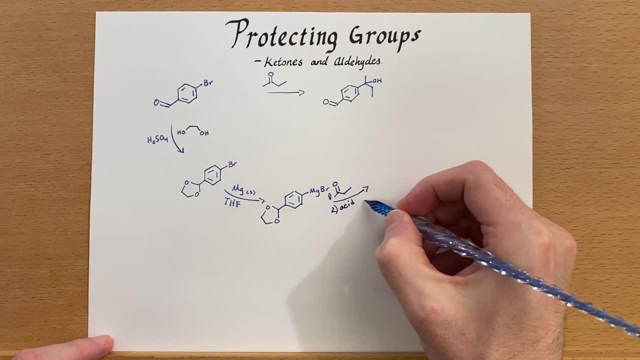 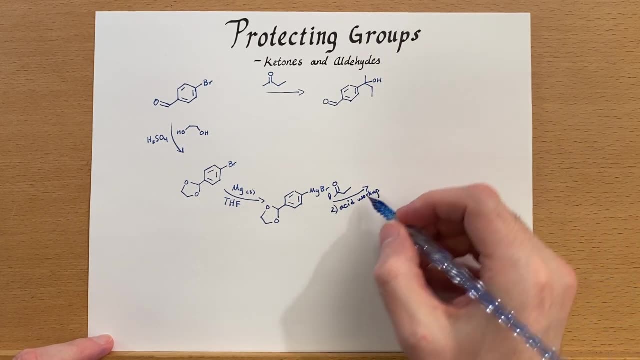 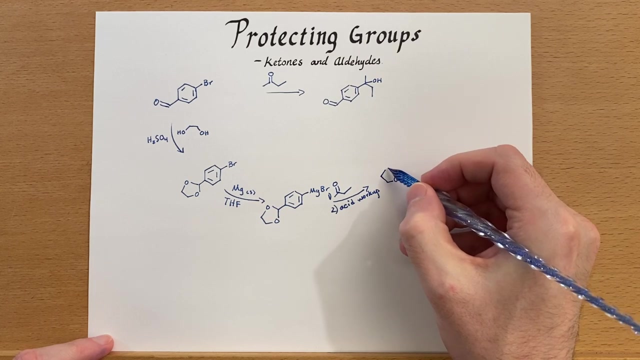 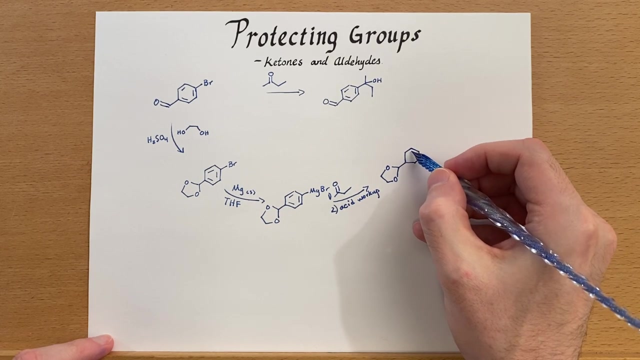 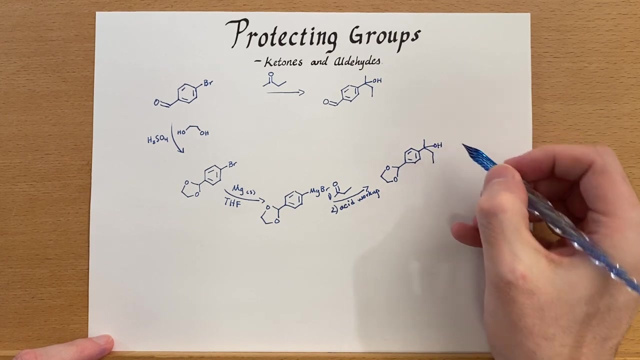 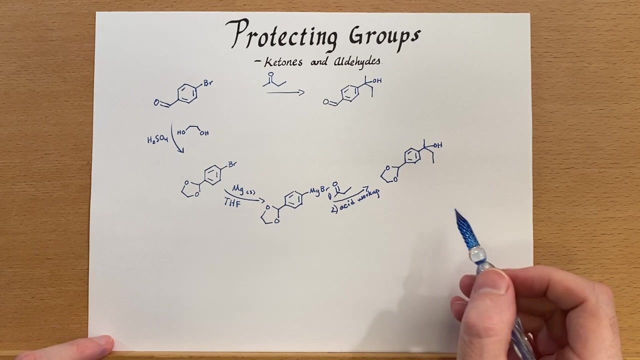 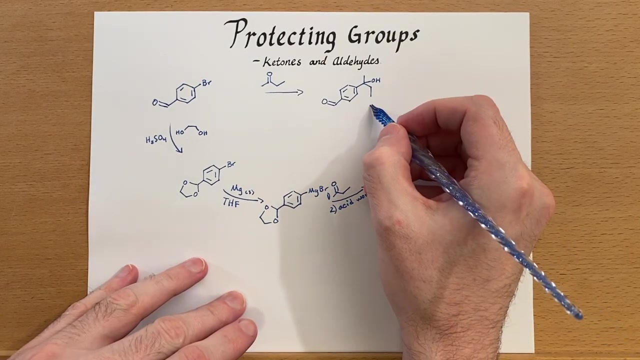 a little acid workup, and let's assume that this acid workup is pretty mild. so we're very close now to our target molecule. at this point, all of our we need to do is de-protect the aldehyde. So in order to do that, we will just add: 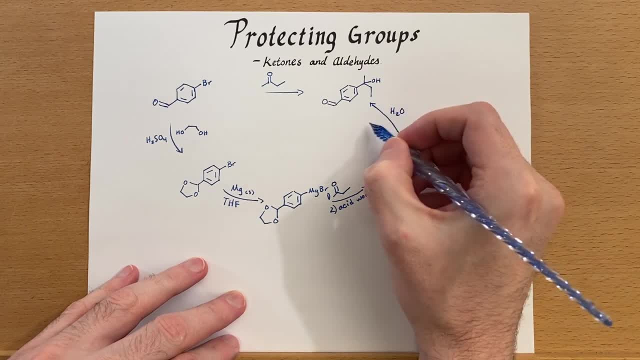 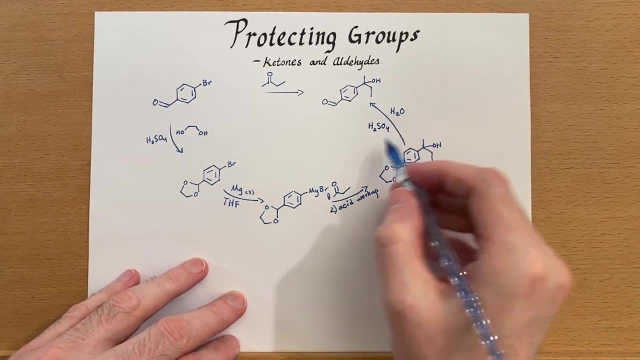 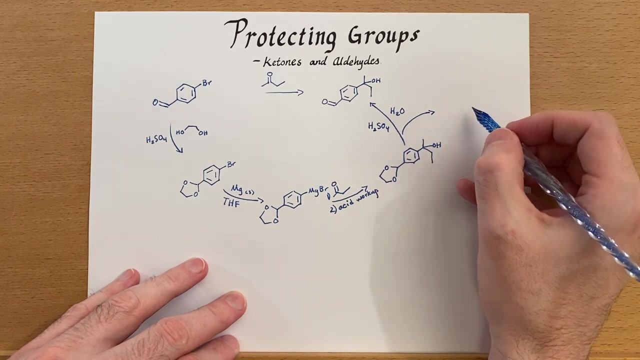 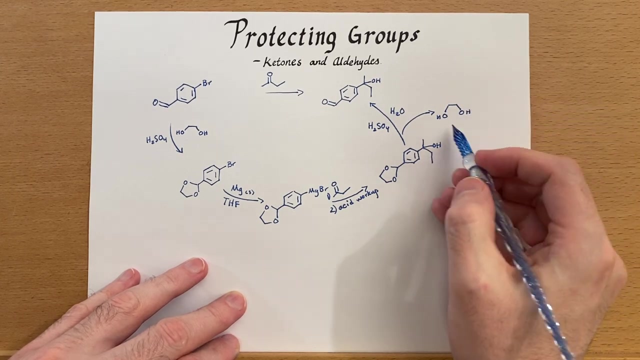 lots of water and a little bit of sulfuric acid. This will remove the ethylene glycol, So I should just draw. maybe I'll draw another arrow over here. This is leaving, We'll get our ethylene glycol back. Yeah, that's kind of a. 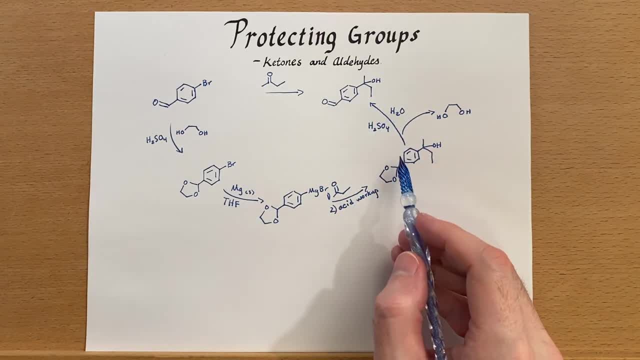 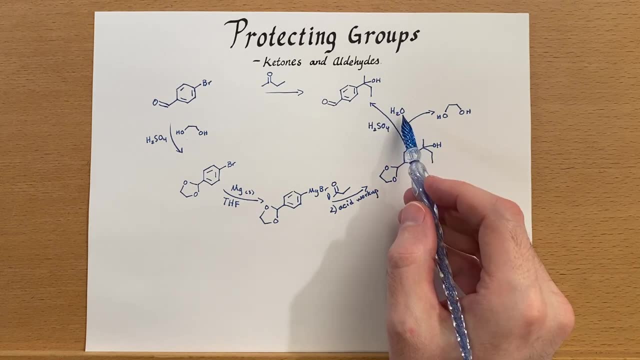 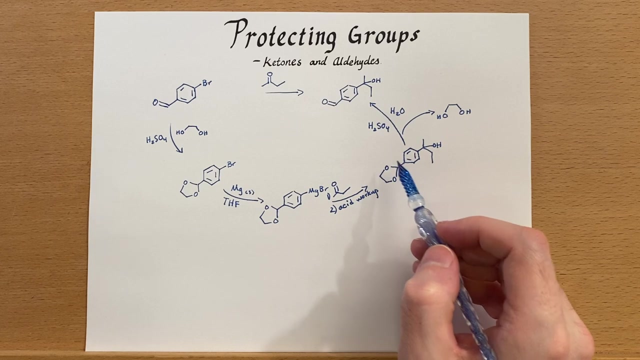 byproduct there And really this is an equilibrium, but we can control that by making sure that we have excess amounts of water and that will tend to drive this equilibrium towards our product. So when we're looking at protecting groups in general, we need them to go on fairly easily and we need them to come. 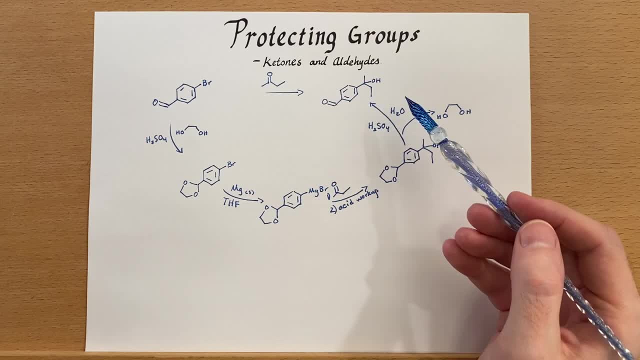 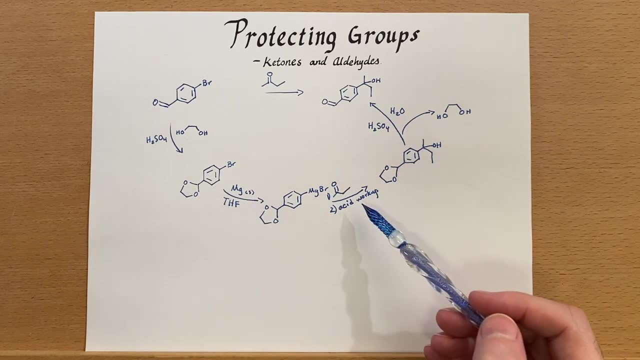 off reasonably easily, But in the meantime we will need them to stay for whatever other conditions that we have. So those are the characteristics that we would like for a protecting group. In this case it's very good protecting groups because an acetal effectively is an ether and ethers are fairly not reactive. 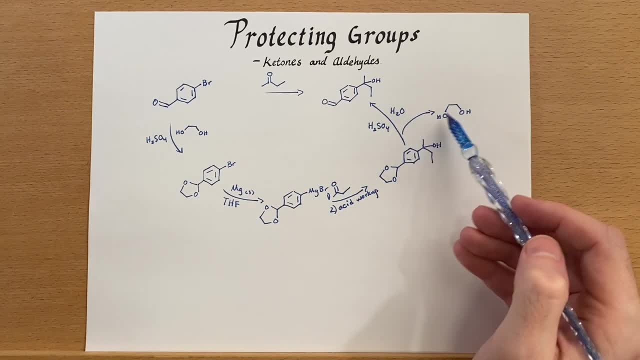 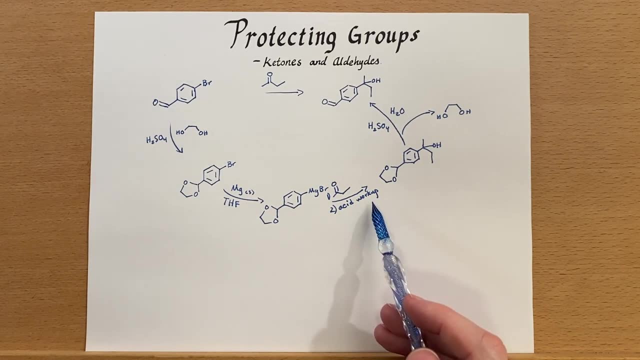 and so it will only come off when we want it to. Now here I did say mild acid workup steps, but I suppose if we wanted to try to do this all in one step and go right to there, we could probably de-protect during that acid workup step just by selecting our conditions appropriately. 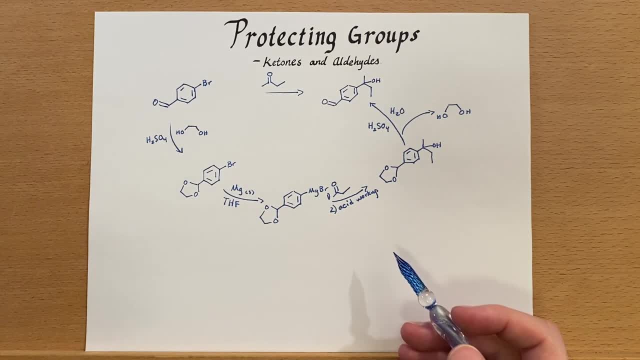 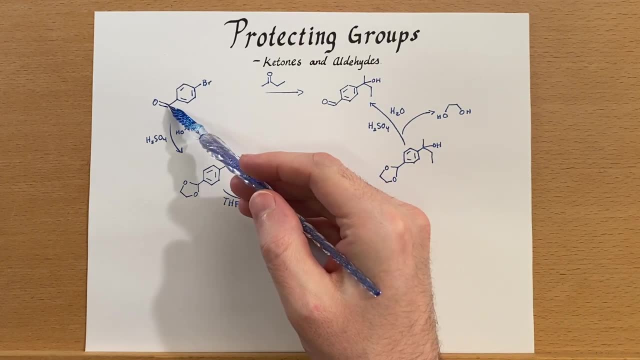 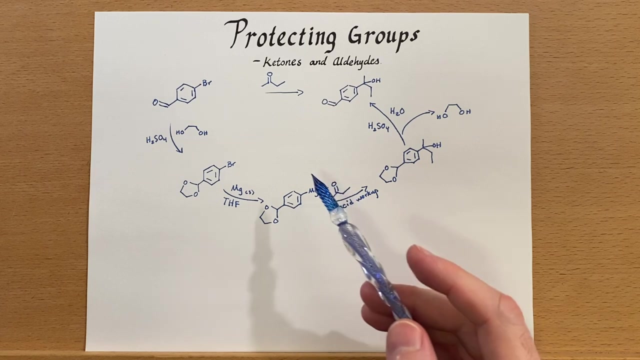 Perhaps right, You'd have to try that out. So this is the standard idea behind a protecting group: We identify a group that we need to protect, we protect it. then we do other reactions that would have reacted with our protected group. 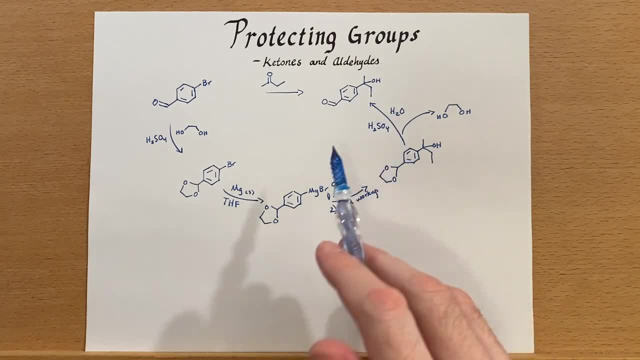 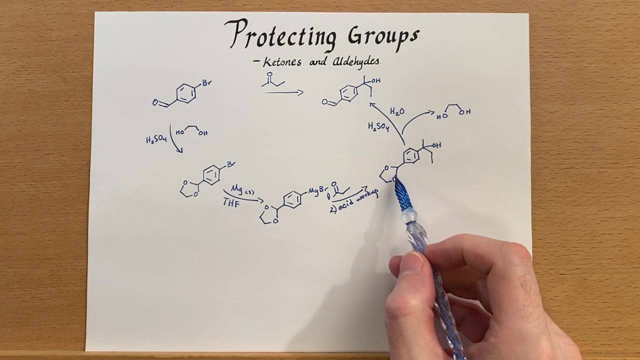 And then later, after we've done all of the reactions that would react with that protective group, then we'll remove it and get to our target molecule. We may wish to keep the protecting group on for quite some time. There might be several steps that we leave that on Or, in this case, we may wish to take it off immediately after. the protecting group And then later, after we've done all of the reactions that would react with that protective group, then we may wish to keep the protecting group on for quite some time. There might be several steps that we leave that on Or, in this case, we may wish to take it off immediately after. 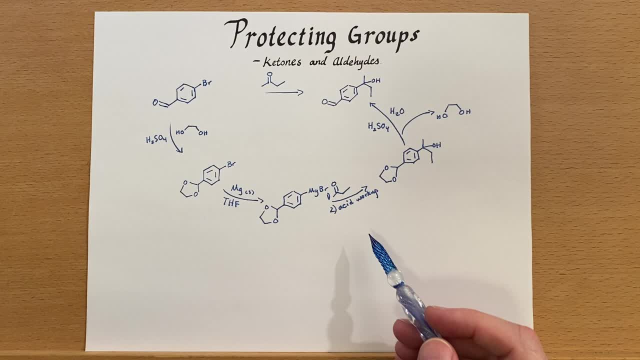 we have the steps that that group is sensitive to. You'll just have to see what makes sense Now. previously, we had designed synthesis so that we would avoid needing protected groups because we hadn't discussed these yet. This allows us greater flexibility in how we design.